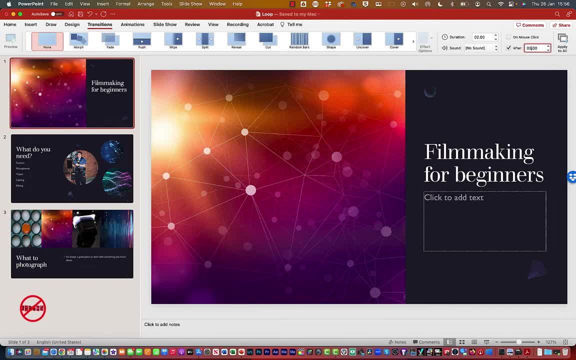 I actually put that in earlier, But I could change it to something else. I could change it to back to two, because what I want to do is just show this to you. I'm not really too bothered about it being on screen for a long time, but I want you to see how it works. I would like it to be just a fade. 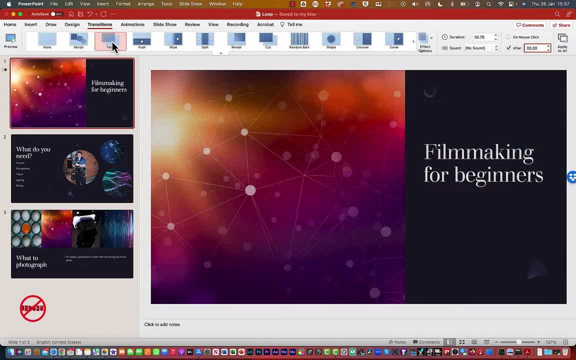 from one slide to the other, And when I clicked on that, you can see it. This gave me a sample of what it looked like. Now I'd like to do the same for all these other slides, So what I'm going to do is over here on the right hand side. it's got apply to all. 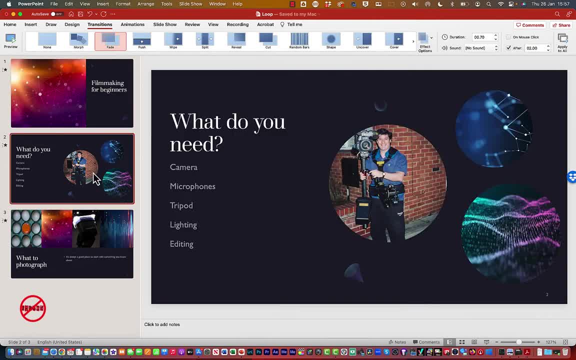 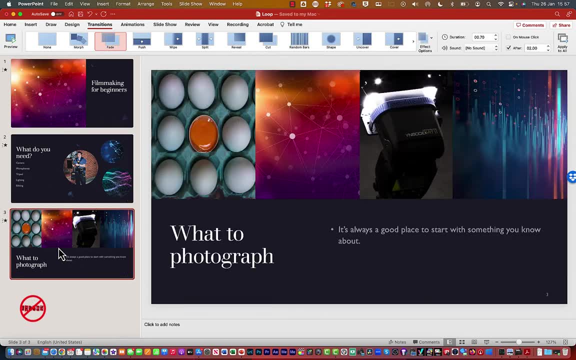 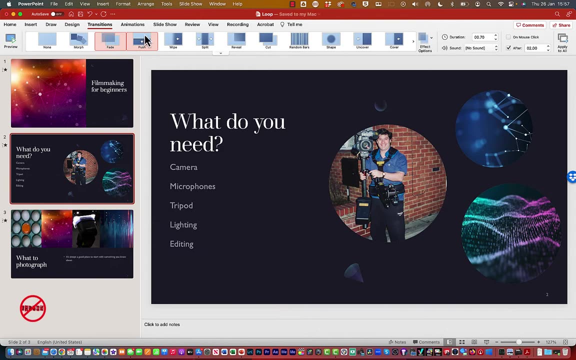 Let me click on that Now. if I go to the next slide, you'll see it's got the fade option. It's got the after two seconds. And let me just check this third slide here And you can see again it's on fade. Now I could go here and change them. I could come to this second one here. 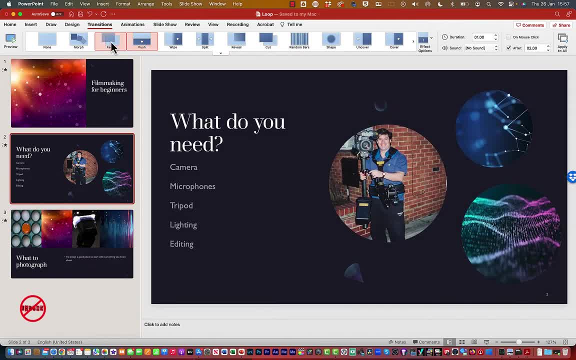 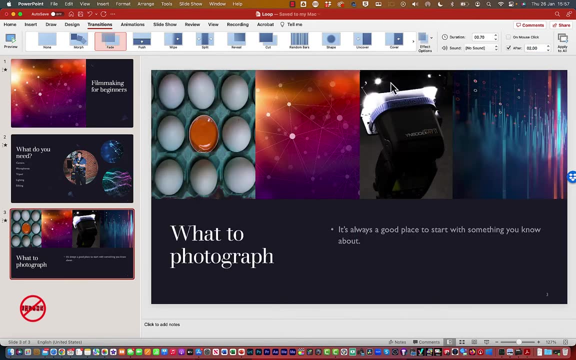 I could change it to a different transition if I like, But I'm going to stick with the fade. It's got a little bit more information on here, So I'm going to make this one three seconds. In reality I might make that longer. Let me just press enter. And this final one here: 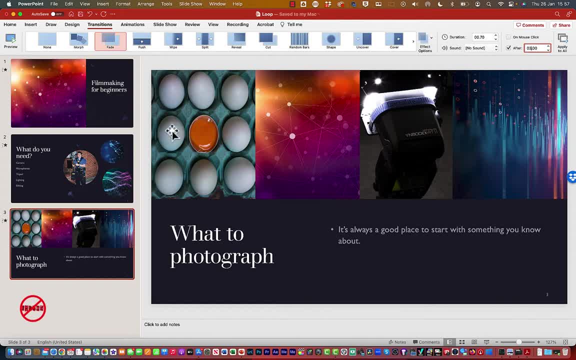 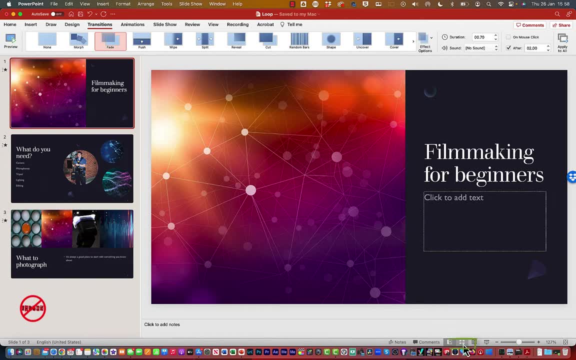 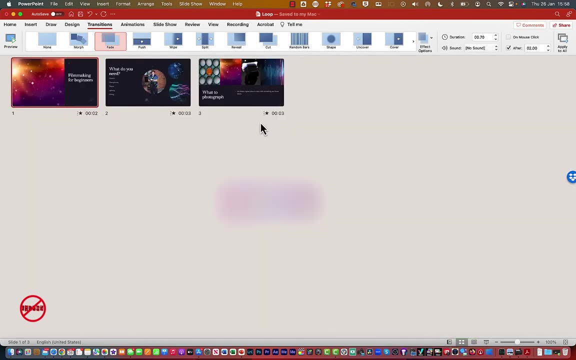 I might just change that to three seconds as well. So there you have it. They are all my slides. Now I could go to my slide sort of view down in the bottom corner here Down at the bottom. If I click on that it looks like a grid. You can now see the timings on there. 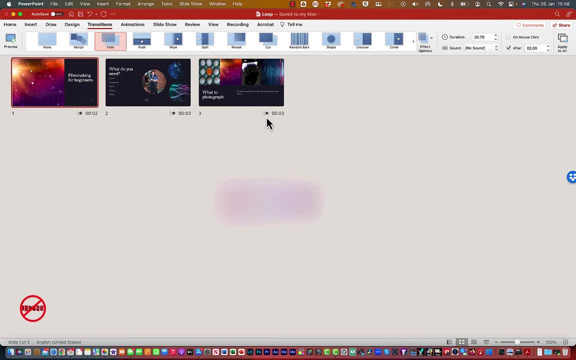 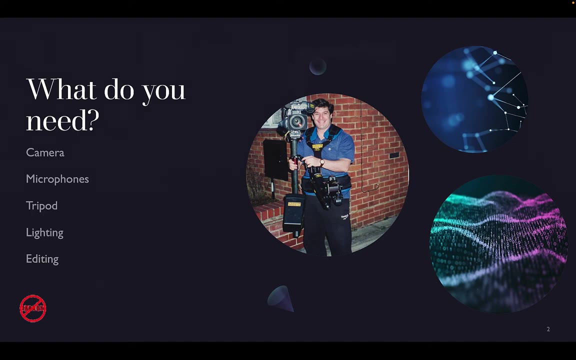 And you can see that it's got this star with some lines to indicate that there's a transition on there. If I was to click on the slideshow- play it- It will go through the slideshow, doing exactly what I said it would do, Which is go from one slide to the other. The only thing is it's got. 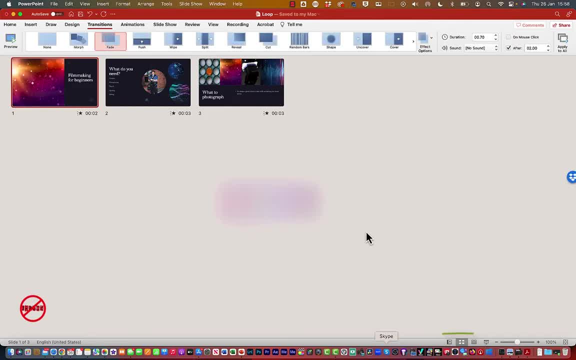 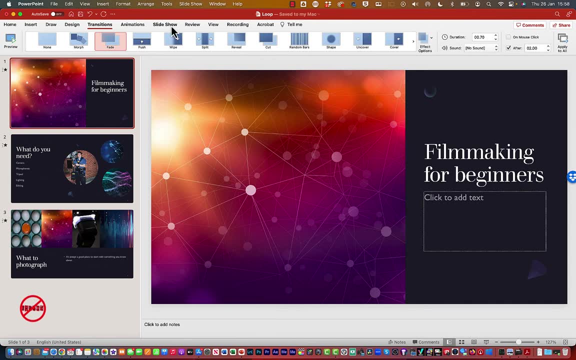 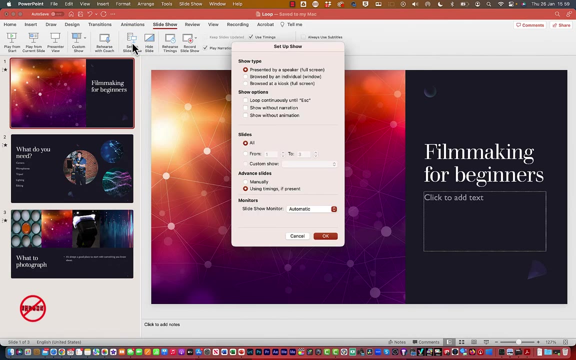 to the end of the slideshow. So let me just end the show there. I'm going to go back to my normal view And over here in my slideshow at the top I'm just going to click on that. You've got a button here for setup slideshow And the thing you need to do here is click on loop continuously.